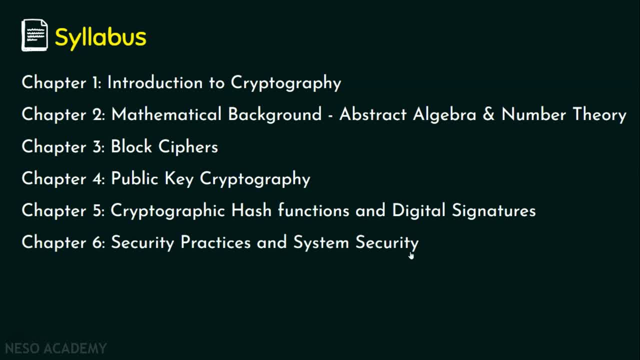 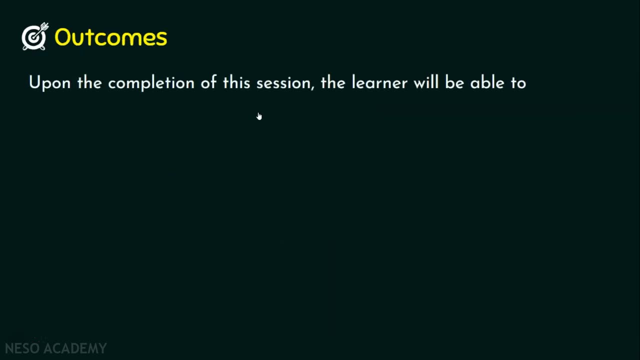 security practices and system security. And finally, in chapter seven we are going to focus on the email security, IP security and web security. Let's start the first lecture, the introduction, Before we step into the topic, we will see the outcomes first. Upon the completion of this session, the learner will be able to: 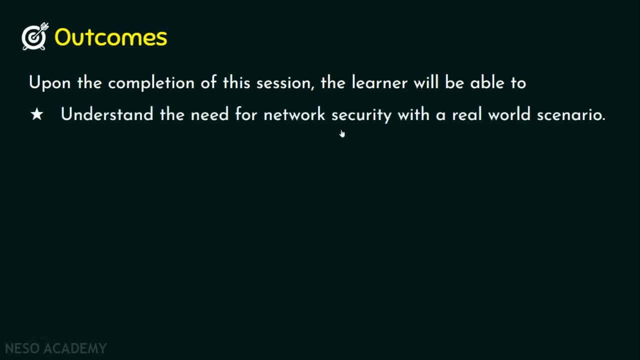 outcome number one: we will understand the need for network security with a real world scenario. And outcome number two: we will know various intentions of attacker. Let's dive into the need for network security. The internet, undeniably an inevitable entity of this contemporary world. 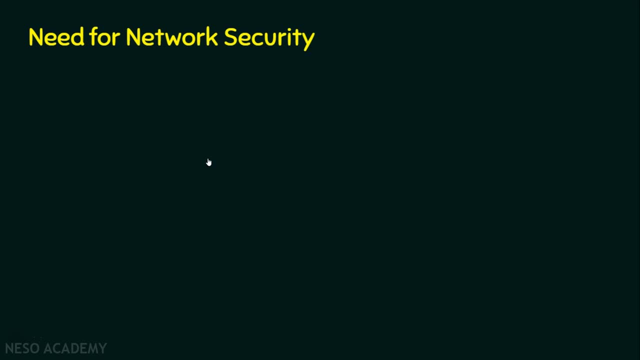 We have both good guys and bad guys on the internet. I mean good guys are legitimate people, Bad guys are attackers and hackers. If you want to carry out any job on the internet, obviously the data should come out of your device first, whether you work with your laptop or you. 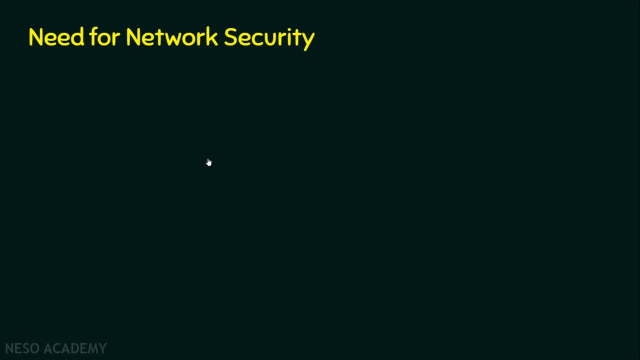 work with your mobile phone whatsoever, But still the data must come out of the device. Once the data comes out of the device, it is obviously. it's not in our hands. We don't know where the data is going to be flowing. We are ultimately relying on the internet to have a sophisticated living style. 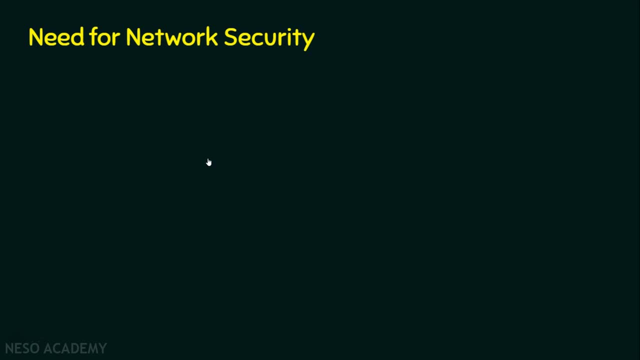 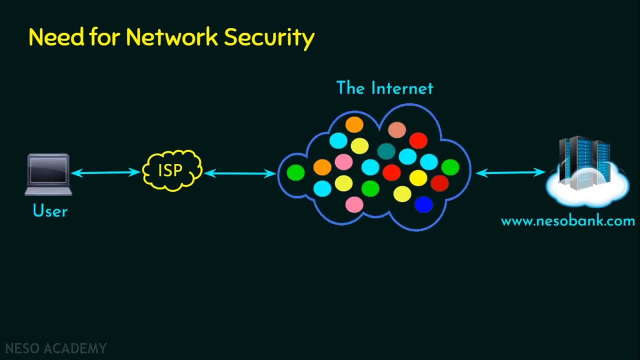 But, as mentioned, we have both Good guys and bad guys. We don't know what the bad guys are going to do with the data that we are sending, So we need to understand why security is important In order to understand why do we need a network security. 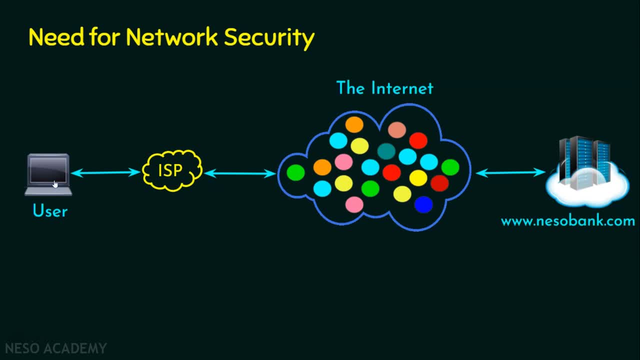 we will take an example. Say you are working in this computer and you are going to do some financial transaction with nesobankcom. It means you are having an account with nesobankcom and you are going to do some fund transfer, for example. Obviously, we are relying on the internet to accomplish this task. 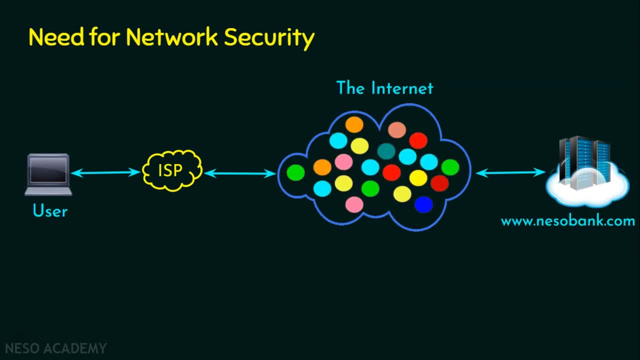 The internet is a public network which contains all kinds of people. If you are a legitimate user, you cannot expect everyone to be legitimate, as like you, Because we have attackers in the real world scenario. What the attacker is going to do on the internet? The attacker only can answer this question. Attackers may steal data. they may steal 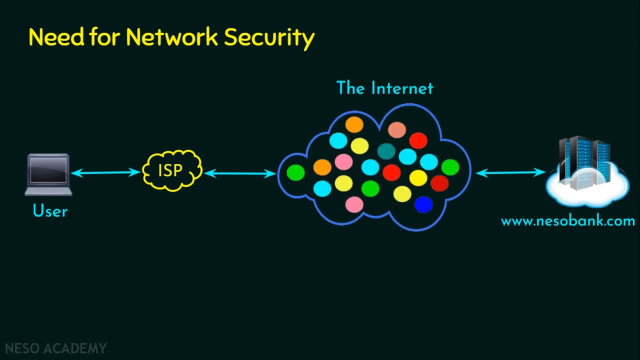 infrastructure. they may steal reputation. they may seek ransoms. they do denial of service. they steal, they exploit data more. Only attacker can know for what purpose he is launching an attack. So there are many goals and intentions for an attacker on the internet. We all agree: attacking needs intelligence. 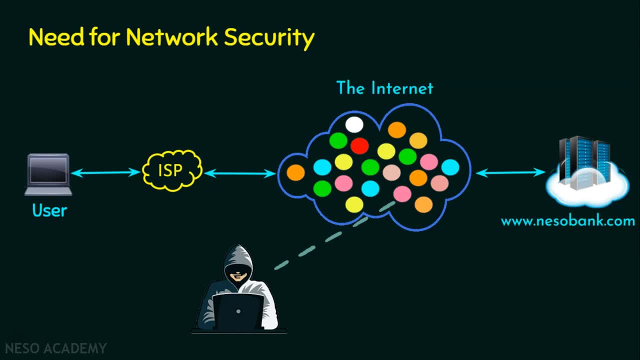 and attackers are intelligent people. But it's waste to blame the attackers, because we should focus more on protecting our data and protecting our infrastructure, protecting our network, protecting our entire system from attacks. Attackers intention will be always launching attacks, But we need to prevent that attack. we need to protect our network. 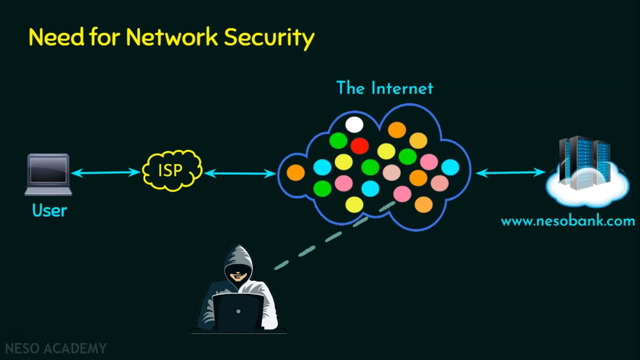 so that we can be safe. We should not be a victim of any such attacks. So what we need to do is we need to protect our data. But unfortunately, once the data leaves our computer system, it is not in our hands. So what we need to do, We need to ensure that the data 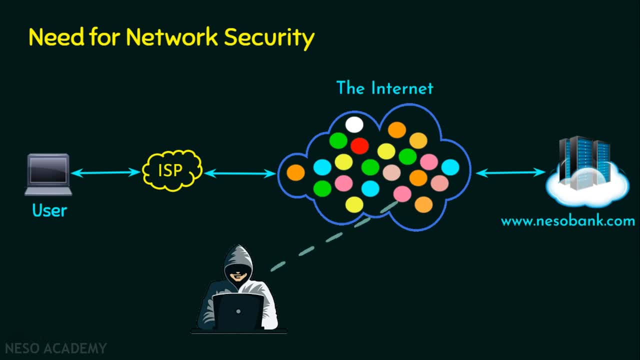 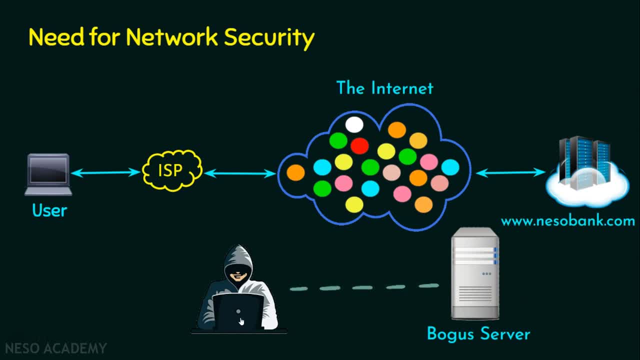 do is we need to protect our data. So what we need to do is we need to protect our, and what this attacker is going to do is he is going to advertise this bogus server in the name of nesobankcom. 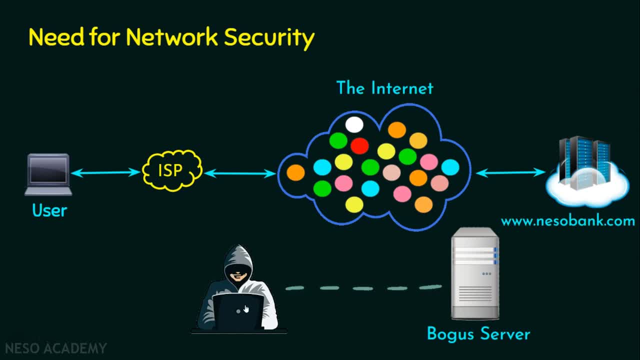 Let's say you are receiving this email, which is advertised by this attacker, and you see the hyperlink is having the title wwwnesobankcom. and what? if you click on it, It will not be going to nesobankcom, rather, it will be going to this bogus server. 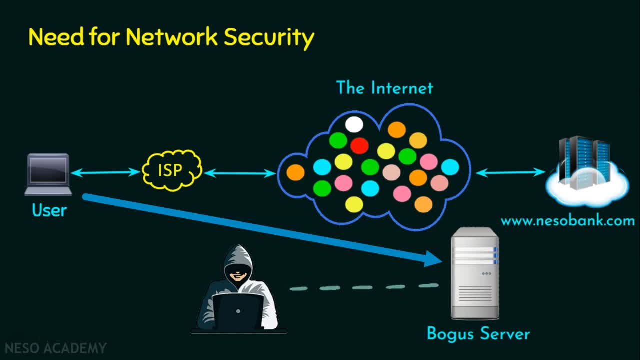 What if you start giving your confidential information to that Gone? It is not being captured by nesobankcom server, which is the legitimate server. Rather, it is being captured by the bogus server. It is actually going to the attacker, The attack. what I mentioned here is an example of phishing attack. 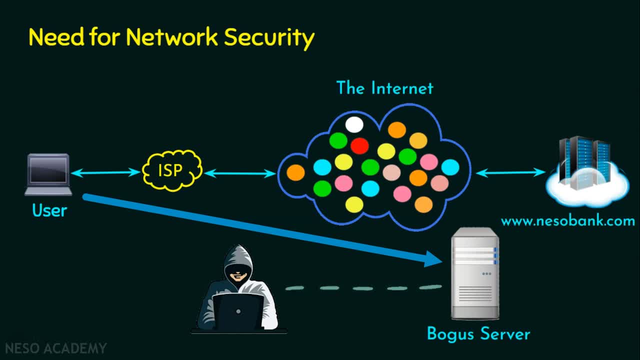 So don't worry about the terms phishing, attack or any other attacks. if I mention We are going to demystify a lot of attacks in this subject. But anyway, we need to be very careful about these attacks because as computer professionals, we should not be a victim of any such attacks.